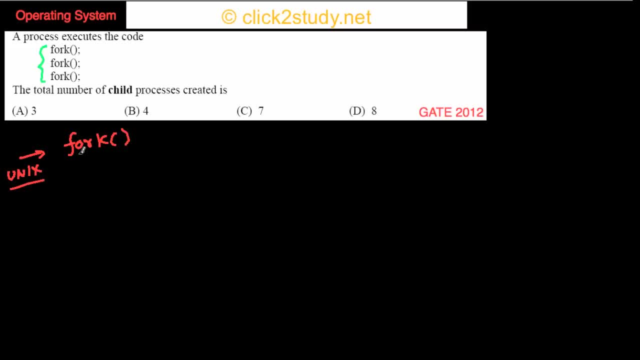 Unix operating system. When a process is running some code and it makes a fork system call- Okay- then what happens is that it creates a child process- Okay, and the child process copies gets the whole code of this process copied into it. Okay, so the code of the child process is the exact copy of the parent process- Okay, and then both of them can run. 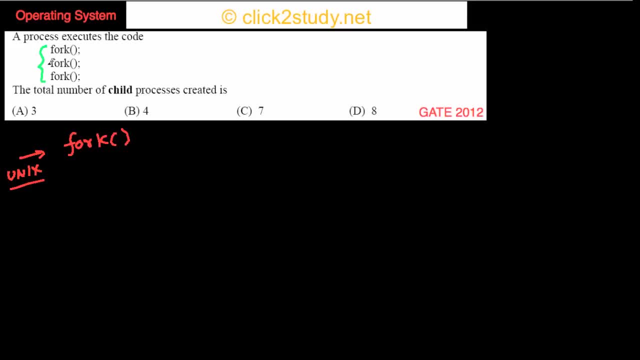 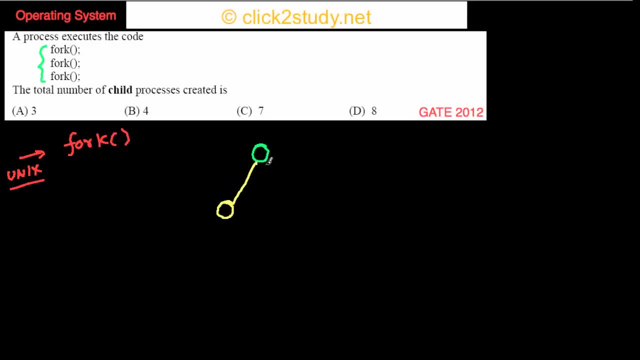 child suppose: okay, and this, the parent continues like this. so when the first for call was made, okay, so suppose this was the first for call. we made the first for call and what we got was a, this child and the parent continued as such. now both this child and both, and this parent as well, there on the same code. 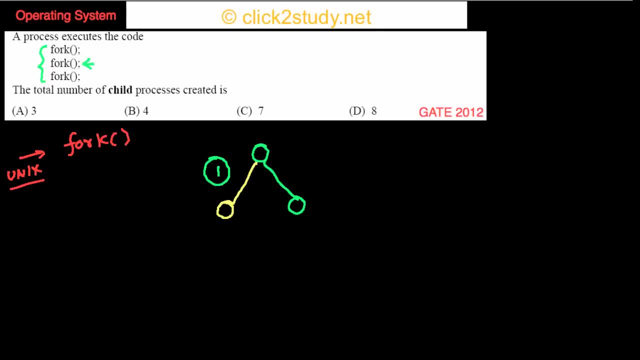 which means now they will run the second fork. so when you will have the second fork on both of them, so this will again have a child like this and this process itself like this, okay, and this thing again, okay. so this is the child and this process. continue that. so I'm making this green and this yellow to make the 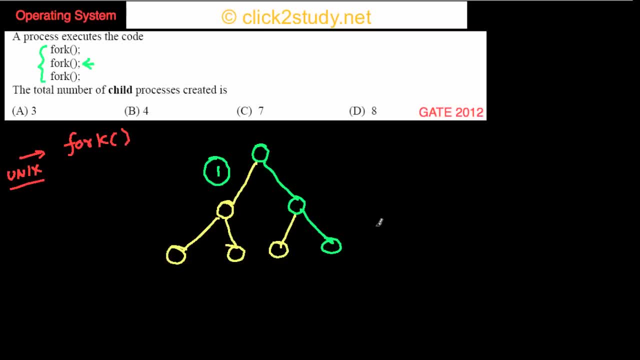 difference that this green is the initial parent process. that continues, okay, and this was done on second fork, and then, if the third fork is made, then you do the same thing for all of them. so you have one more out here like this, here like this, and you have like. 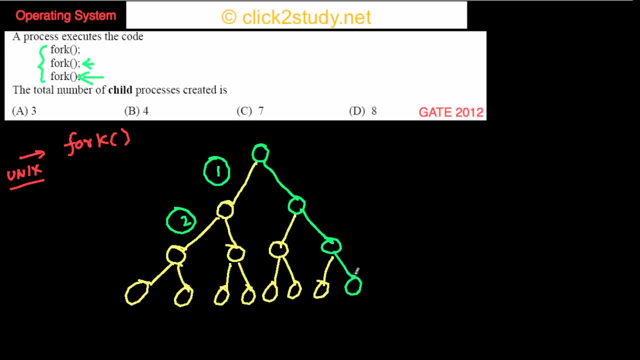 this like this: and the parent continues. and this was on the third fork. okay, so how many you have total processes? so if you look at these leaves, they will give you the total number of processes. there are like one, two, three, four, five, six, seven, eight, but out of these eight, this one is the parent, the parent from the beginning. 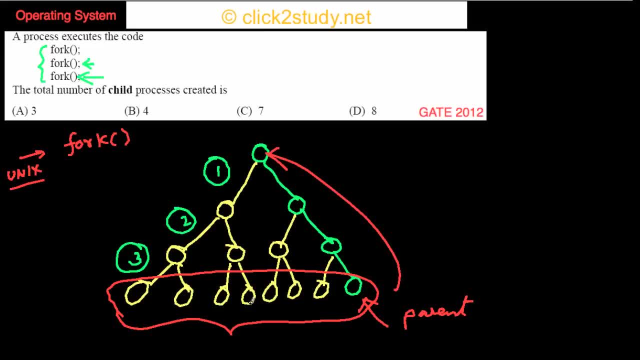 this one. okay, this one is out here. so that means all the remaining are the child processes, which is option seven, and what you can also do is: from here you can get a general formula. okay, if you execute this fork n times, suppose this fork theme is executed n times, so how many processes there will be in total? 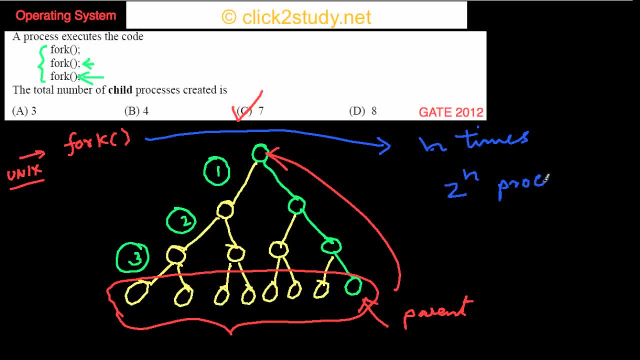 so there will be in total two raised to n processes- okay, and out of these, one will be parent- okay, out of this one will be the parent process, the original one, and the remaining two, raised to n minus one, will be the children processes. okay, or the child processes, and that's it. 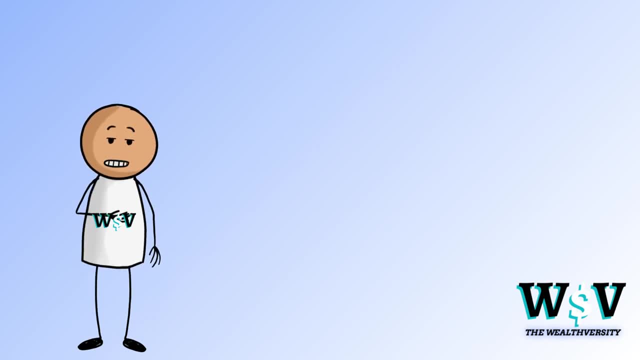 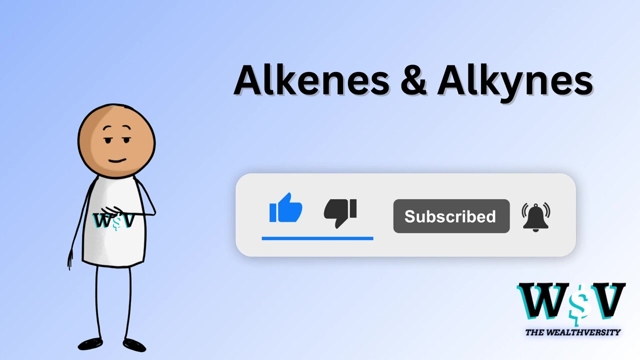 Hello and welcome back to our channel. Today we will be talking about organic chemistry, particularly alkenes and alkynes, and their structures, formulas and properties. Before we start, make sure to like, comment, share and subscribe so you don't miss any of our fun educational videos. 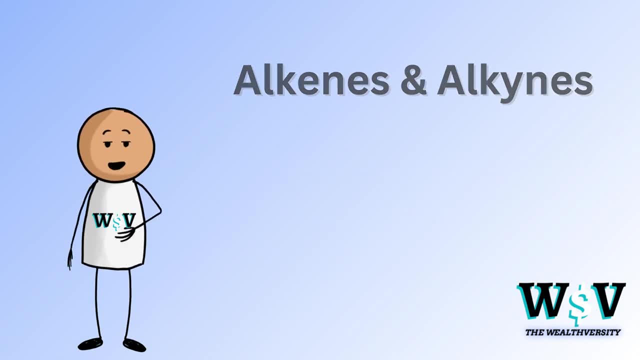 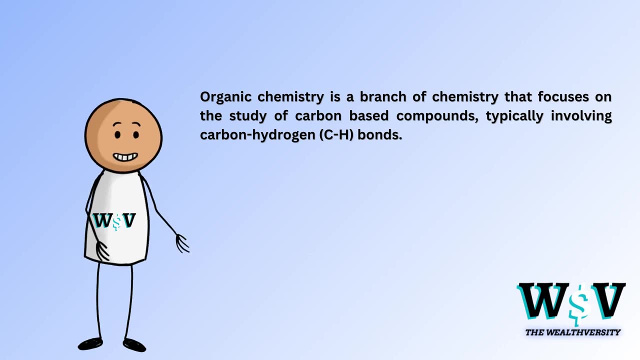 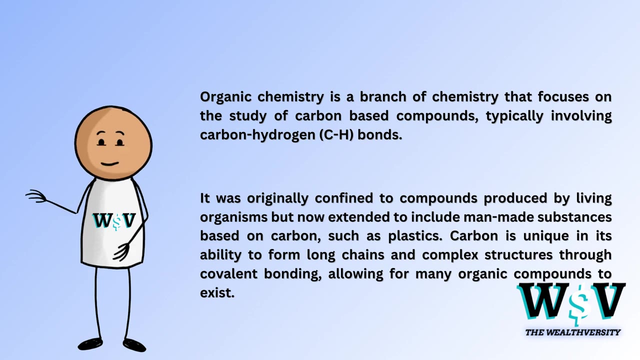 We have previously talked about what organic chemistry is, but let's recap. Organic chemistry is a branch of chemistry that focuses on the study of carbon-based compounds, typically involving carbon-hydrogen bonds. It was originally confined to compounds produced by living organisms, but now extended to include man-made substances based on carbon. 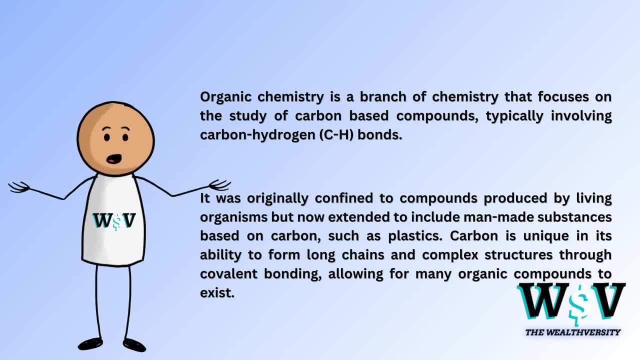 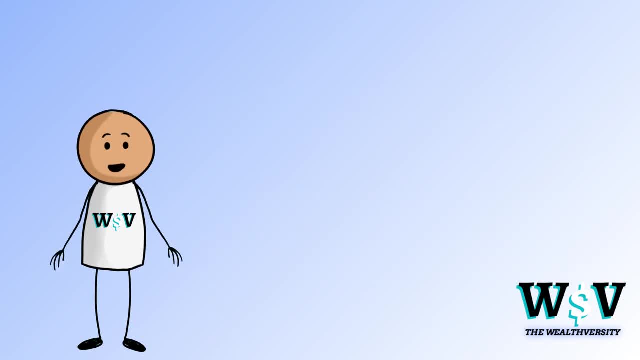 such as plastics. Carbon is unique in its ability to form long chains and complex structures through covalent bonding, allowing for many organic compounds to exist. Now, what are alkenes and alkynes? Alkenes and alkynes are both hydrocarbons. 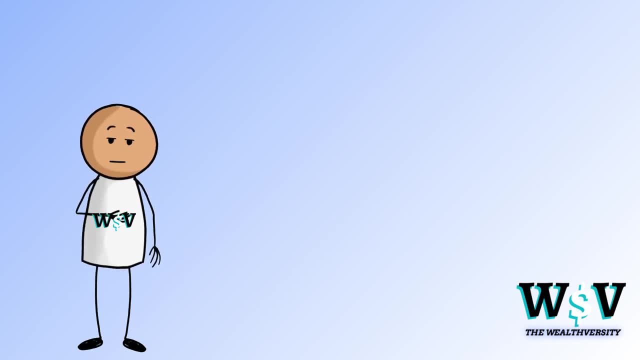 meaning that, just like alkanes, they consist of long carbon chains bonded with hydrocarbons. They are also known as hydrocarbons. Alkenes and alkynes are both hydrocarbons, meaning that, just like alkynes, they consist of long carbon chains bonded with hydrocarbons.